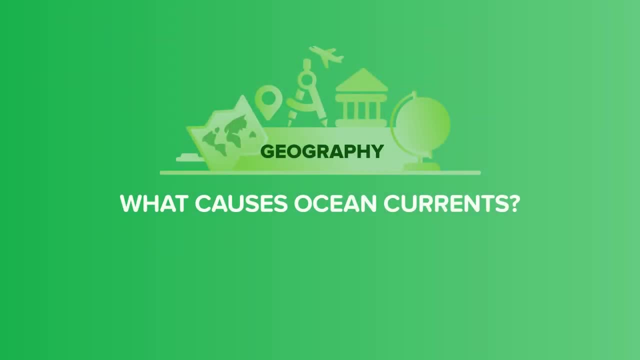 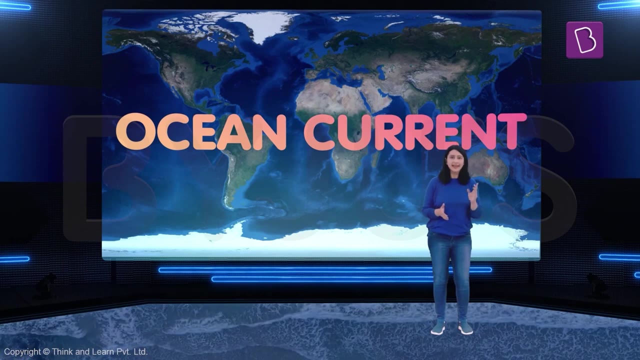 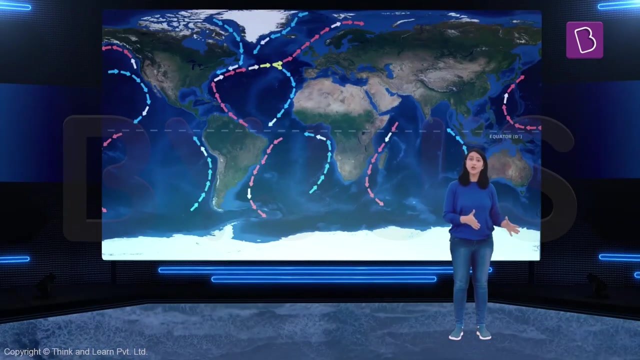 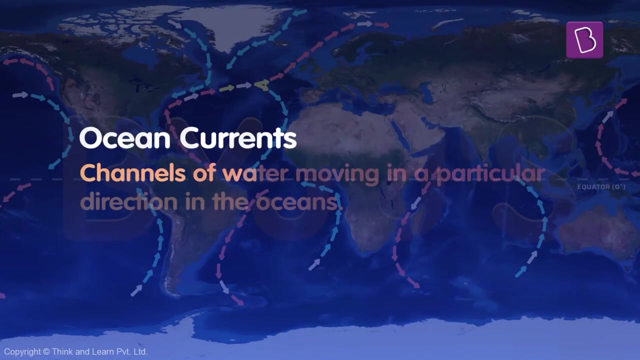 What is an ocean current? Will I get a shock from it? Hey, no, an ocean current is something else. It is like a river inside an ocean, A path of sorts. That's right. Ocean currents are channels of water moving in a particular direction. in the oceans, Now, we are all quite familiar with moving. 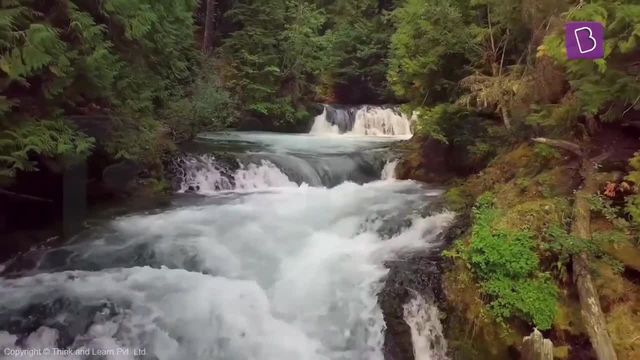 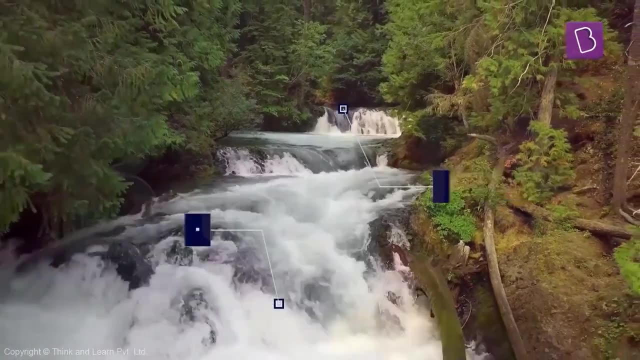 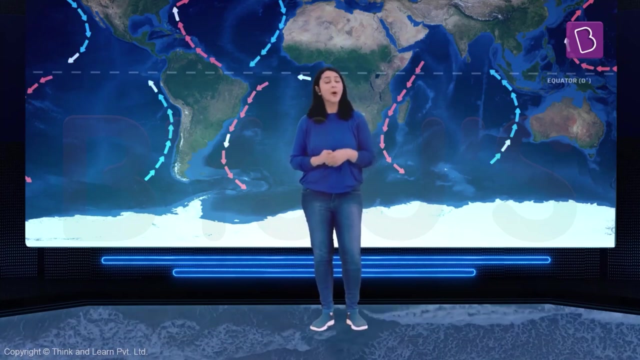 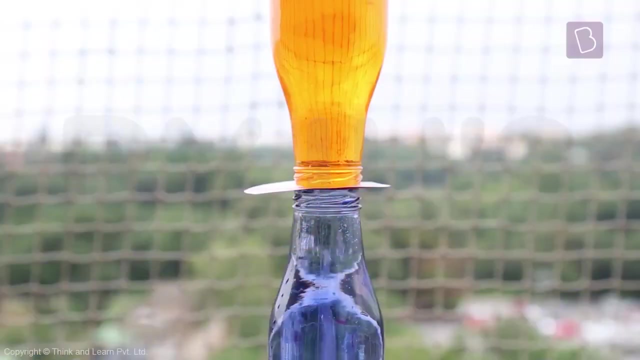 water like streams and rivers. We know that they move, because water moves from a higher region to a lower region. Pretty standard. But is this the same reason for ocean currents? What do you think? Look at this experiment. We have two bottles here, One filled with blue cold water and the other filled 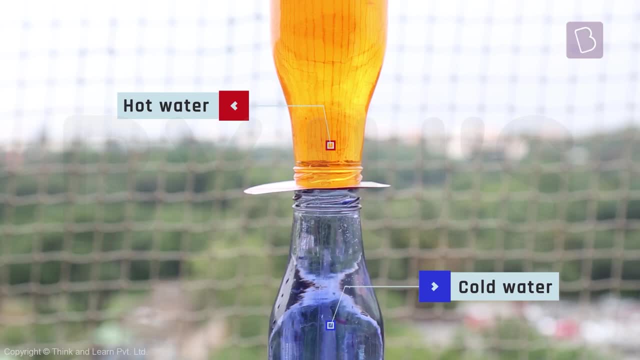 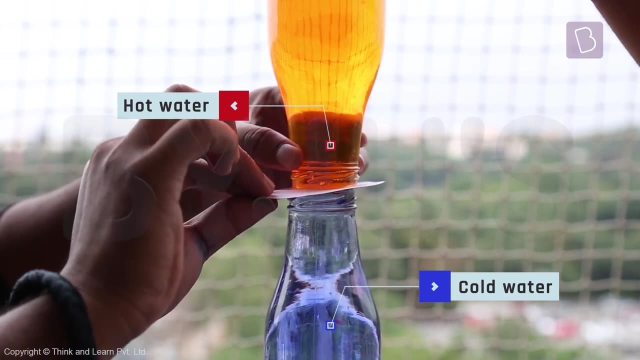 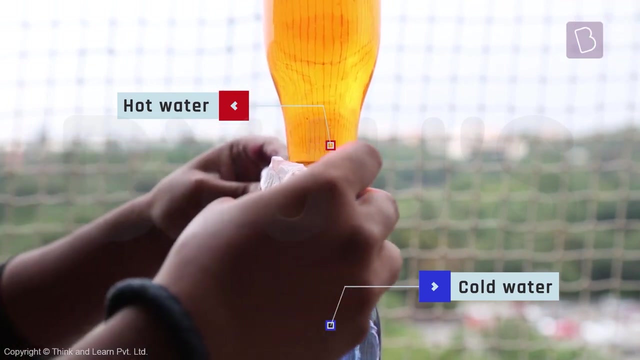 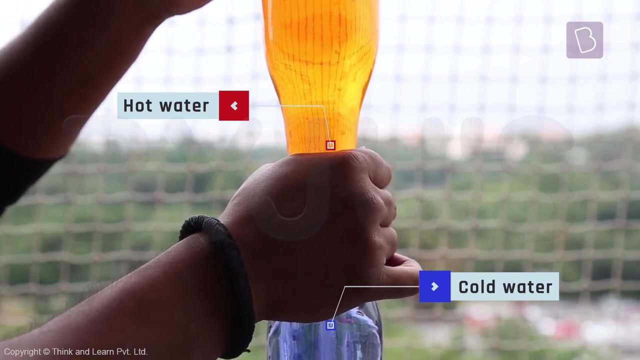 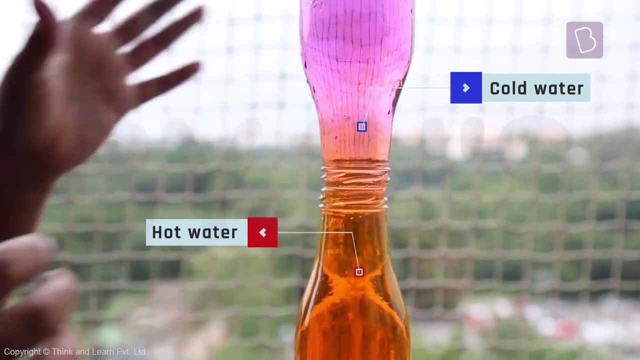 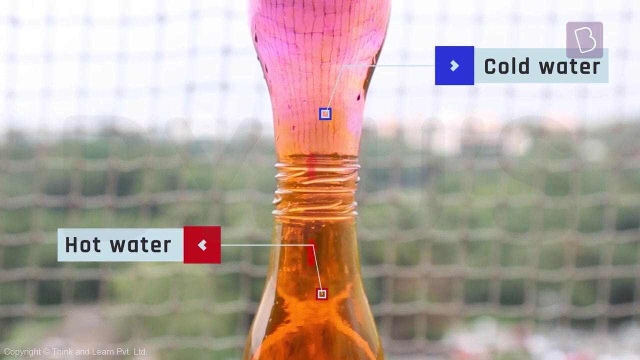 with red hot water. Watch what happens when both of them come in contact with each other. Look closely: The warm water is flowing up and the cold water is flowing down. How cool is that Turns out. this is the sea water. How cool is that Turns out. this is the sea water. How cool is that Turns out. this is the sea water. 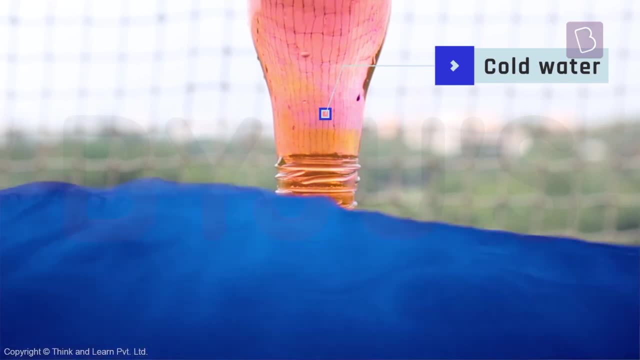 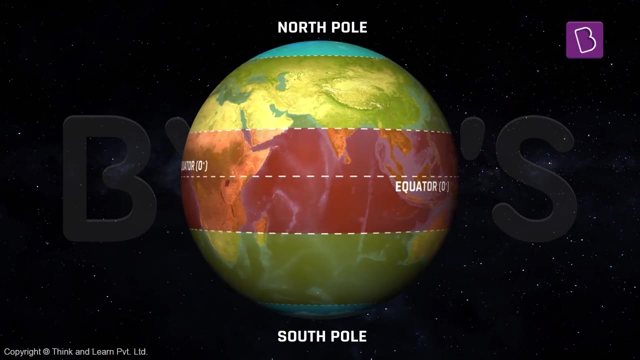 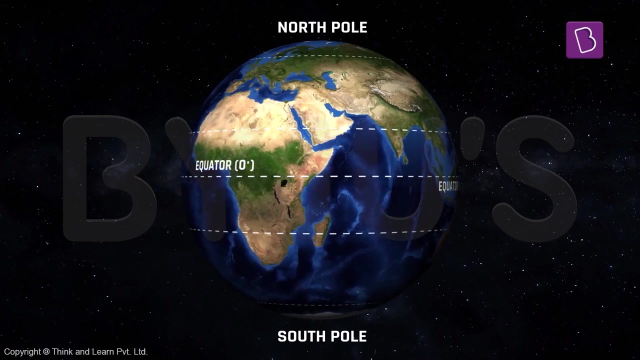 This is the secret of the ocean currents too. By now we know that the earth is divided into these heat zones. It's hotter near the equator and colder near the poles. That also means that ocean water is hot near the equator and cold near the poles. 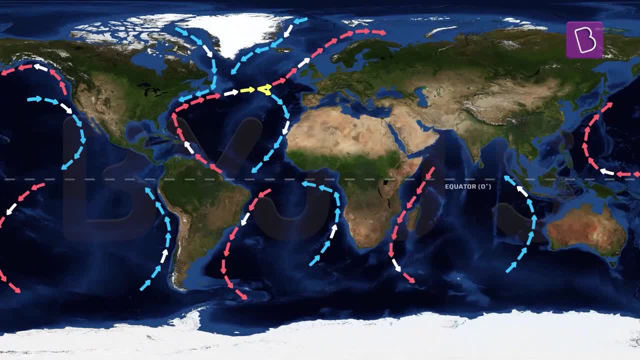 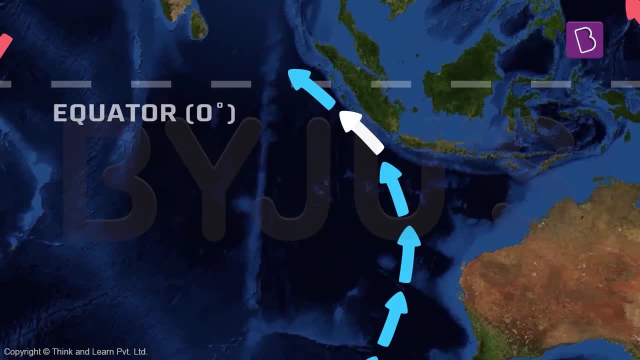 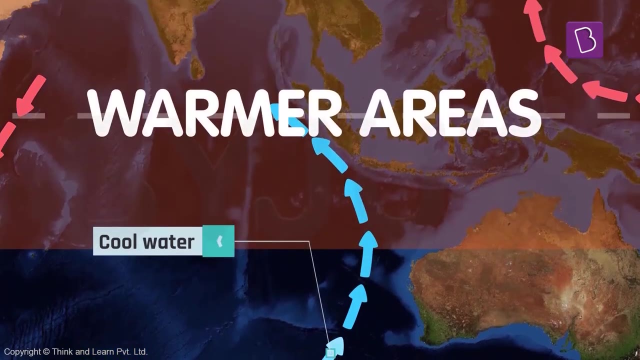 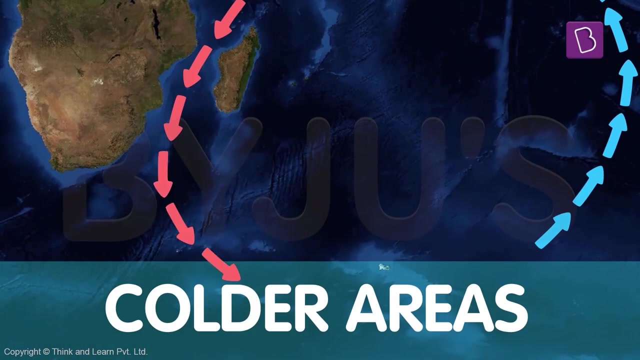 Well, just like in our little demonstration, water is indeed moving from the equator to the poles and back to the equator. This is what ocean currents are: Channels of cool water moving to warmer areas and channels of warm water moving to colder areas.